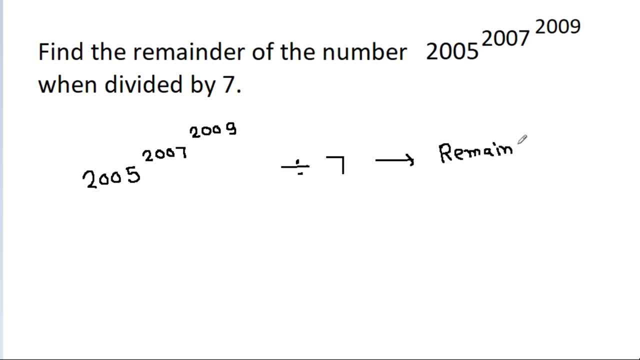 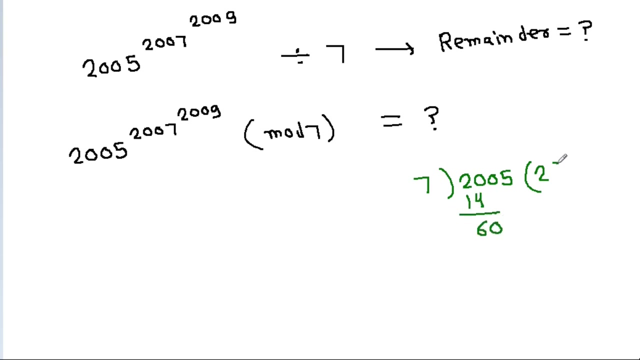 have to find remainder, or we can say that we have to find 2005, power 2007, power 2009, mod 7.. And if we divide 2005 by 7, then it is 2 times 14,, 6,, 0,, 8 times 56,, 4,, 5 and 6 times 42. 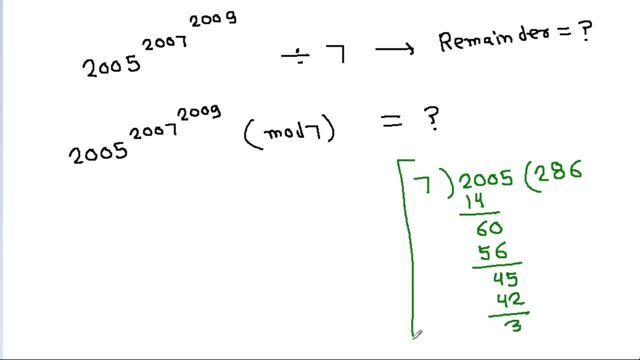 and 3.. So the remainder is 3. That means 2005 is equivalent to 3 mod 7. So 2005 power 2007 power 2009 will be equivalent to 3 power 2007, power 2009.. 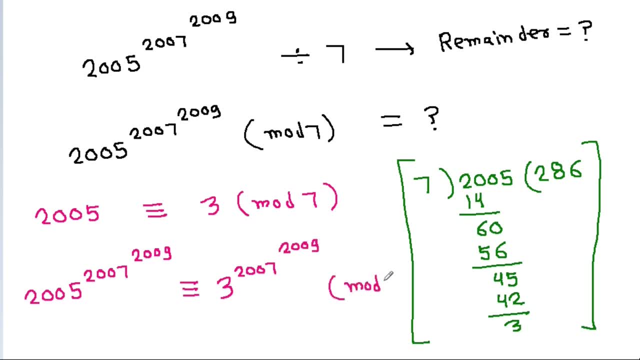 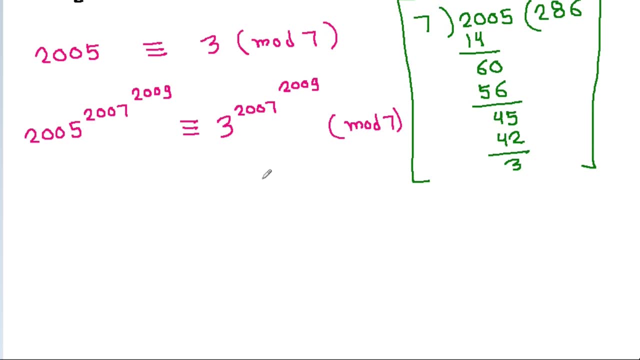 That means 2005 is equivalent to roughly 349 mod 7.. And now we need to find any x, such that 3 power x is equivalent to 1 or minus 1 mod 7.. Because it is easier to denote 1 and minus 1, because we saw that 1 is equivalent to 1.. 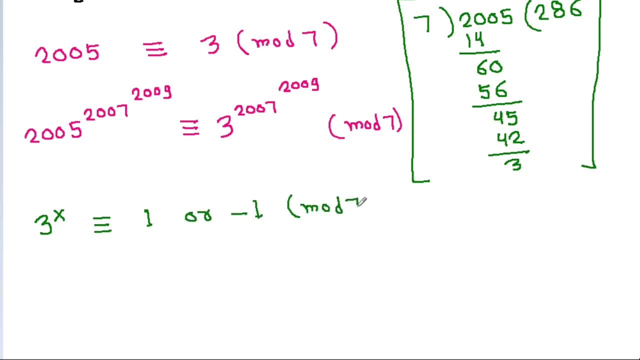 Now we haveIL m electronics equations that we have learned earlier, that are square root of nothing but 1.. And now we have to find ن, seventh power 1. instead of 3, and we can easily think that 3 power 3 is 27, that is equivalent to minus. 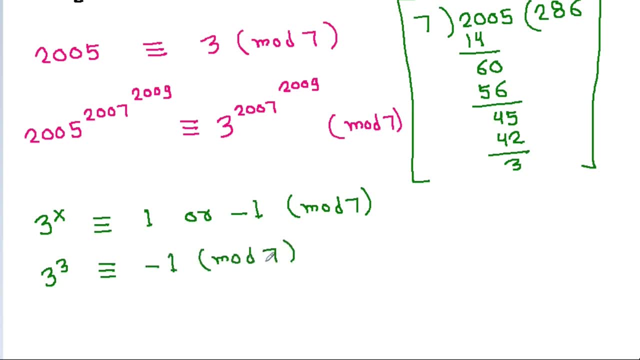 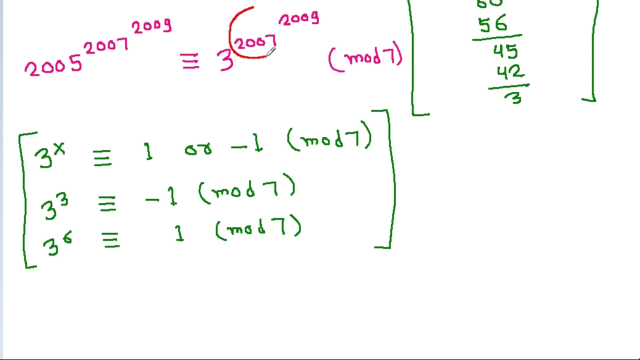 1 mod 7 and I am more comfortable with 1. so if we square it both side, then 3 power 6 will be equivalent to 1 mod 7, and here we have 3 power 2007, power 2009.. So suppose 2007 power 2009, it is equal to 6 mod 7.. 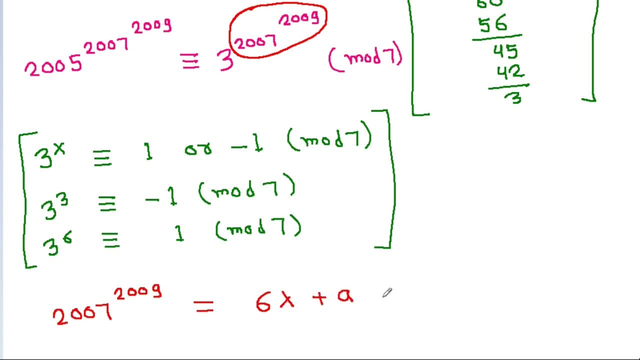 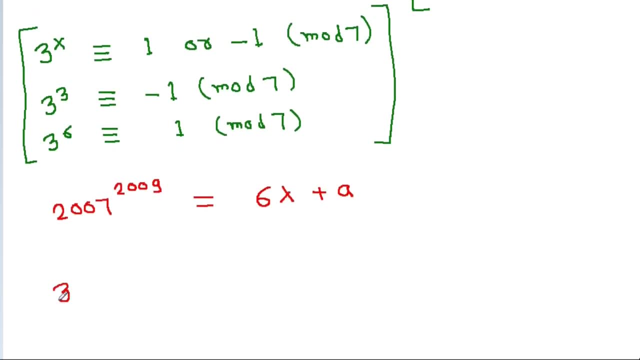 6 times some lambda minus a, Then 3 power 2007 power 2009 will be equal to 3 power 6 lambda minus a, and it is 3 power 6 lambda times 3 power a. So this is 3 power 6 lambda times 3 power a. 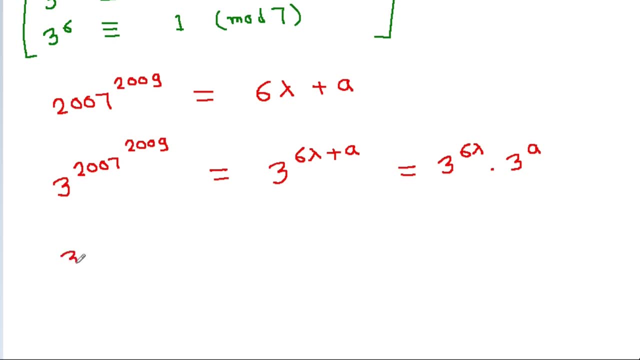 So 3 power 2007 power 2009 is equal to 3 power 6 lambda is 3 power 6 power lambda times 3 power a. So 3 power 2007 power 2009, mod 7.. So this is 3 power 7.. 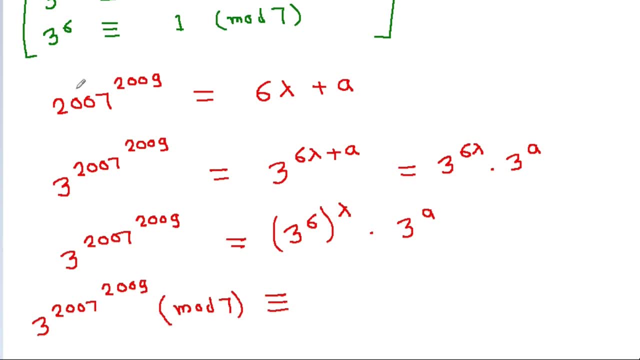 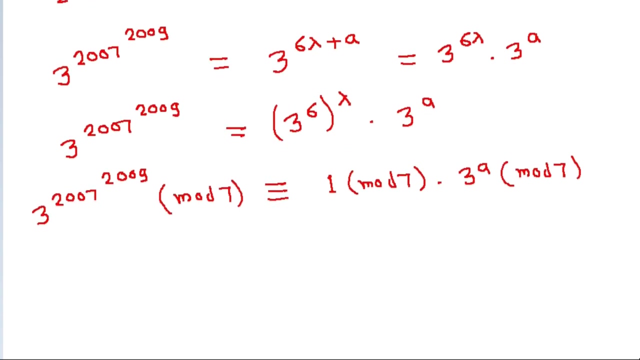 Mod 7 will be equivalent to 3 power 6 is equivalent to 1 mod 7.. So 3 power 6 power lambda will be equivalent to 1 mod 7 times 3 power a mod 7.. So we get 3 power 2007.. 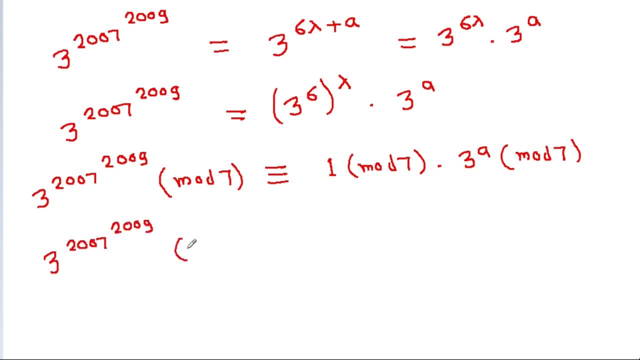 So 307 power 2009 mod 7 is equivalent to 1 times 3 power a is equivalent to 3 power mud 7.. So 3 power 2007 power 2009 is equivalent to 3 power a mod 7.. 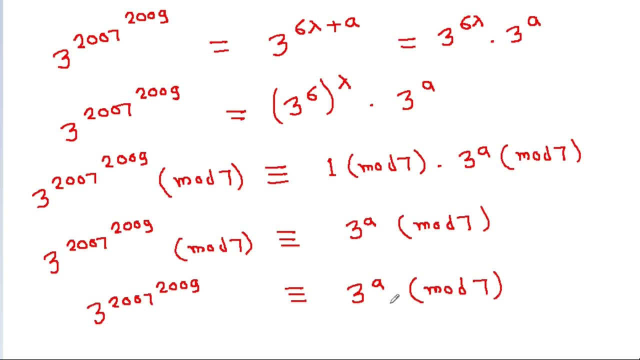 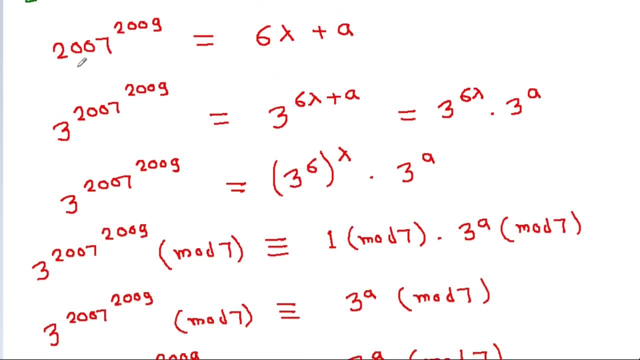 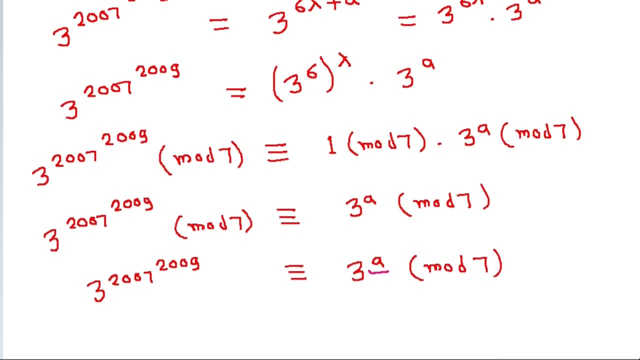 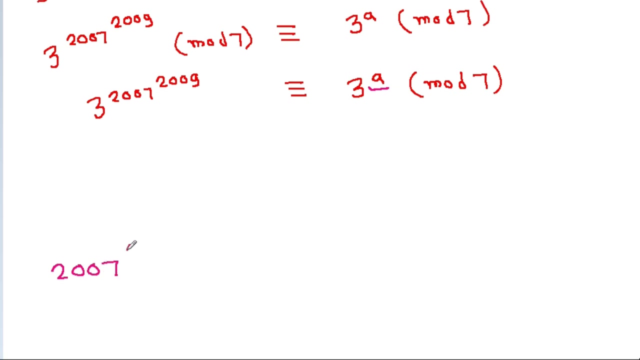 So Now we need to find A and we have 2007 power 2009 is equal to 6 lambda plus A. We have 2007 power 2009 is equal to 6 lambda plus A, So we can say that A will be equivalent. 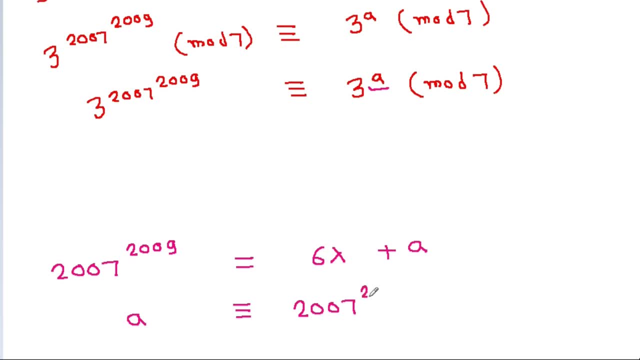 to 2007- power 2009, mod 6.. And if we divide 2007- power 2009, mod 6.. So we can say that A will be equivalent to 2007- power 2009, mod 6.. So if we divide 2007 by 6, if we divide 2007 by 6, then it is 3 times 18, 2, 0, 3 times 18. 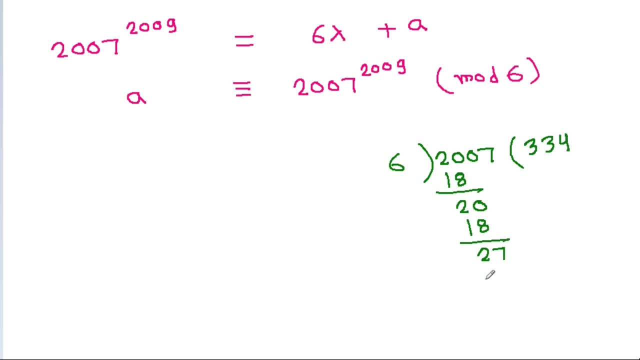 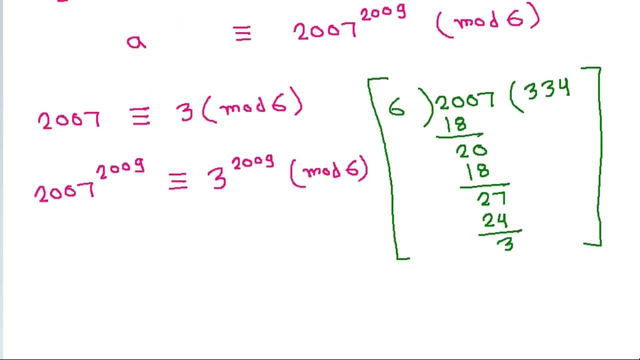 2, 7, 4 times 24 and 3.. So the remainder is 3.. That means 2007.. 2007 is equal to 3 mod 6.. So 2007 power 2009 will be equal to 3 power 2009 mod 6.. And 3. 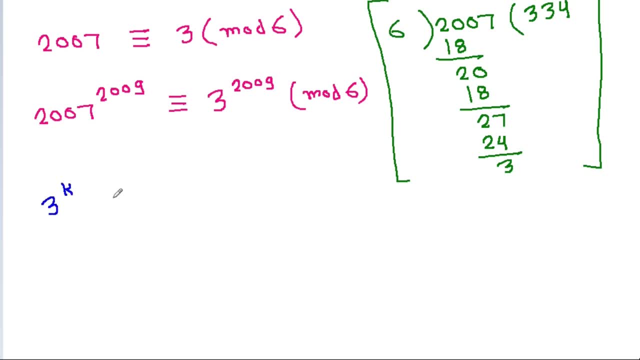 power anything. suppose k. It is equivalent to 3 mod 6.. You can also check it: 3 power 1 is equal to 3. that is equivalent to 3 mod 6.. 3 power 2 is equal to 9, that is equivalent. 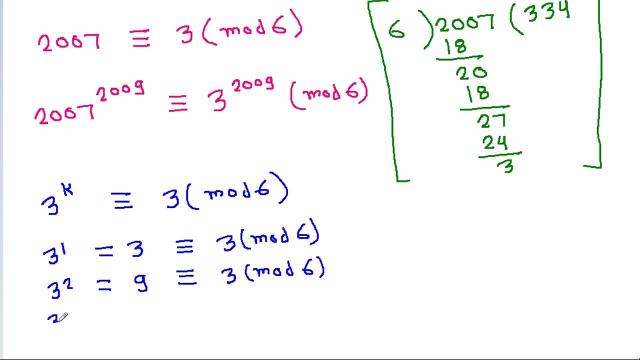 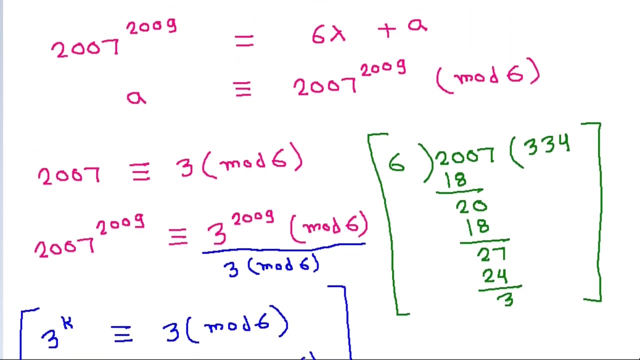 to 3 mod 6.. 3 power 3 is equal to 3 mod 6.. is equal to 27, that is equivalent to 3 mod 6. 3 power 4 is equal to 81, that is equivalent to 3 mod 6, and so on. so 3 power 2009 mod 6 will be equivalent to 3 mod 6, so it is.